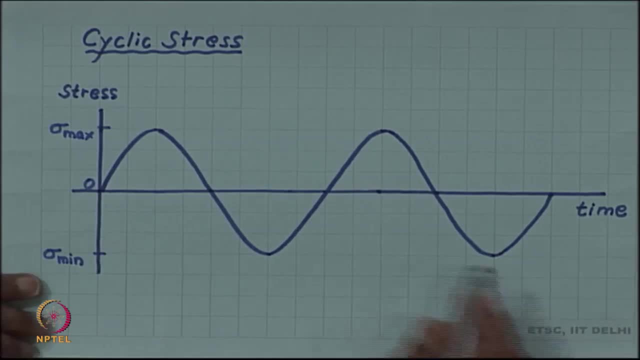 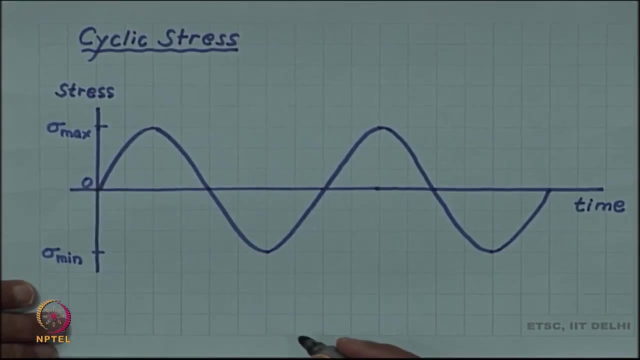 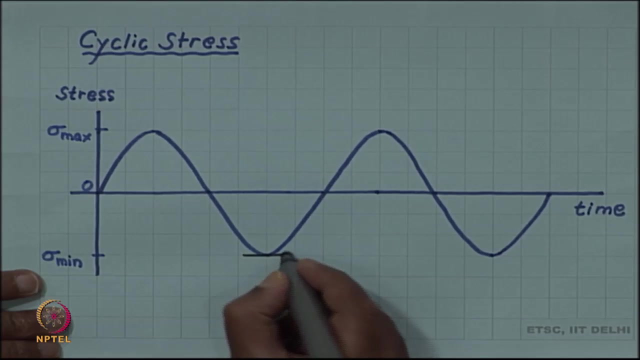 and it is a sinusoidal kind of loading. then we can define several parameters, like the maximum and minimum stress we have already defined, Then the difference between the maximum and minimum stress, this total stress value. this is called the range, this is called the. 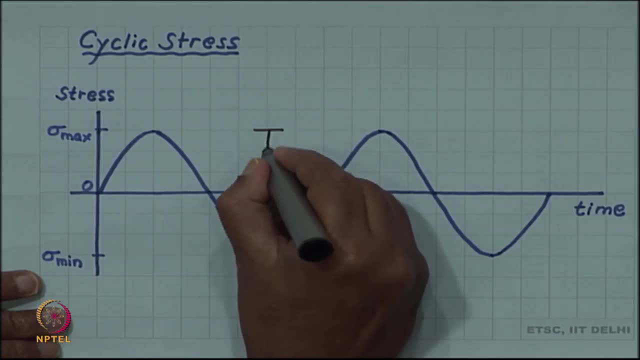 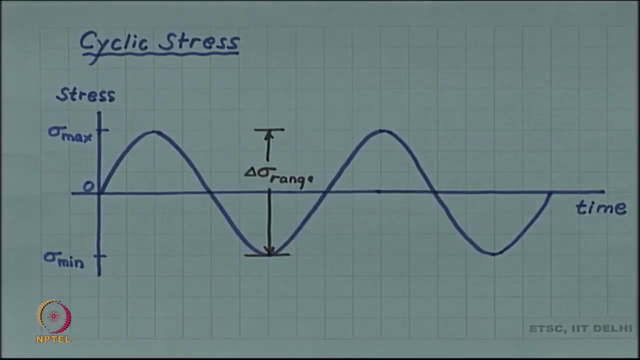 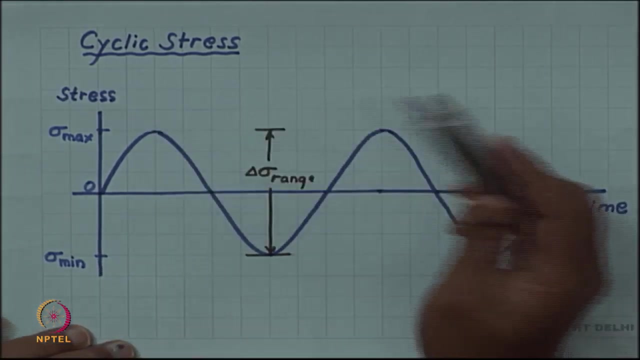 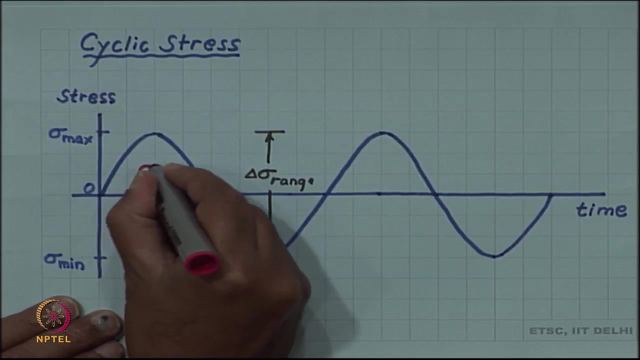 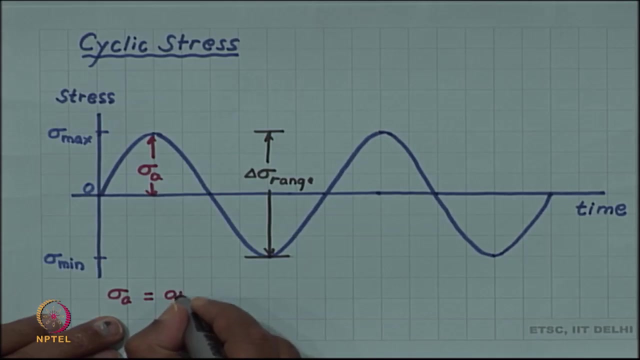 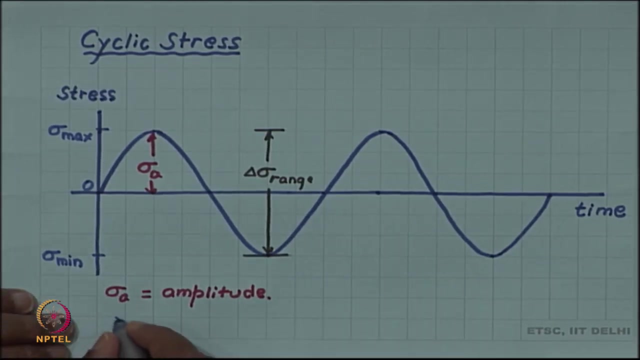 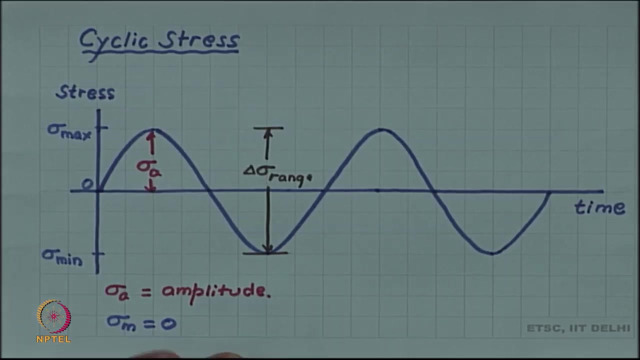 range. this is range, then the value from the mid of the range to the maximum value. that is called the amplitude. So this is the amplitude and the mean value, which in this case is 0 sigma. sigma mean is the mid value here. 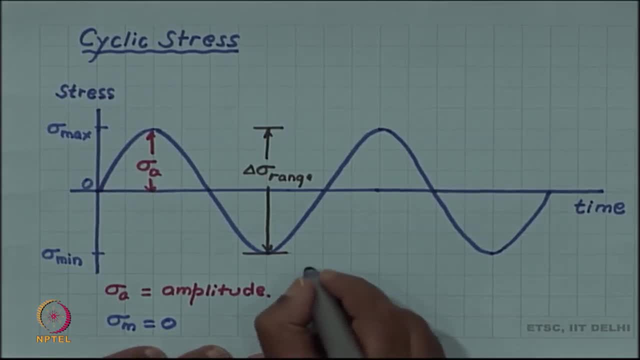 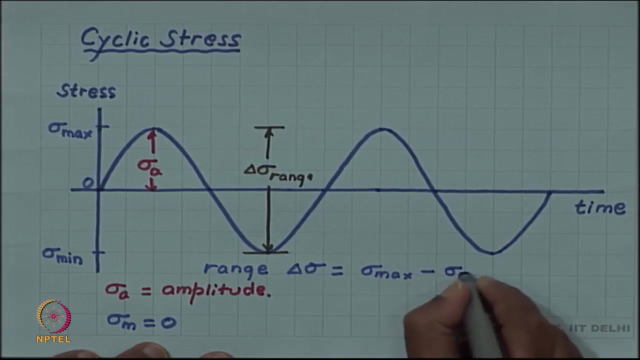 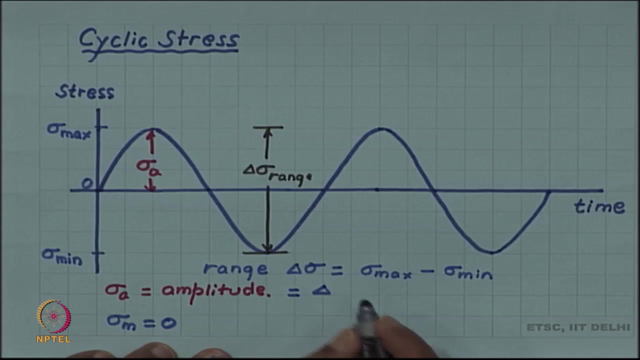 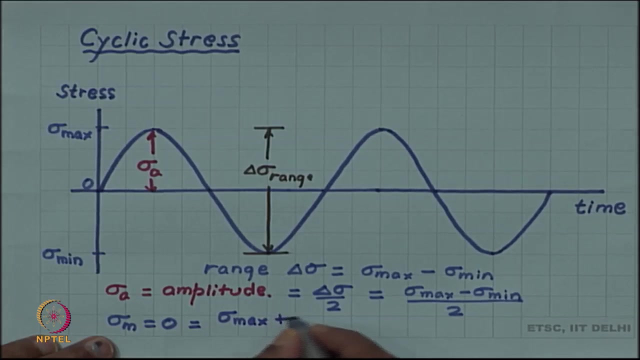 So the amplitude we can define sigma range, delta, sigma, sigma max minus sigma min, and amplitude will be half of the range, And the mean value, which is 0 in this case, is actually defined as the mid value of sigma max and sigma min, which is sigma max plus sigma min by 2.. So this kind of cycle where 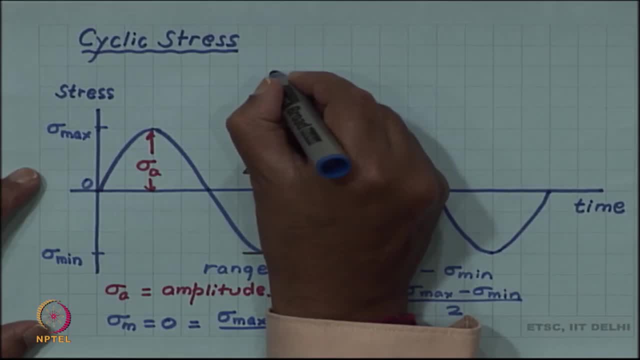 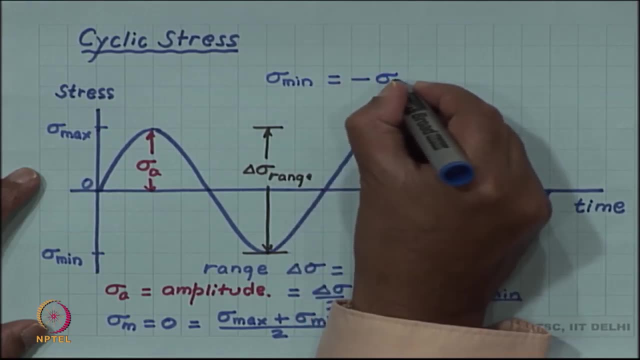 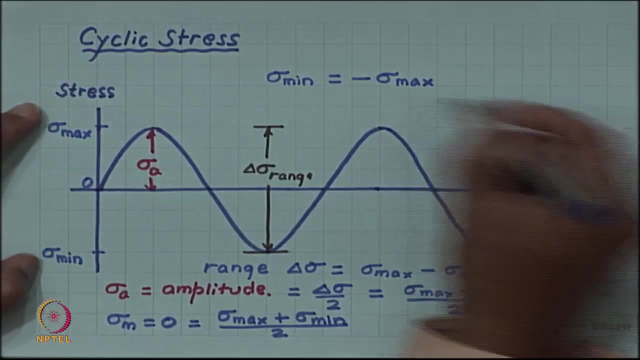 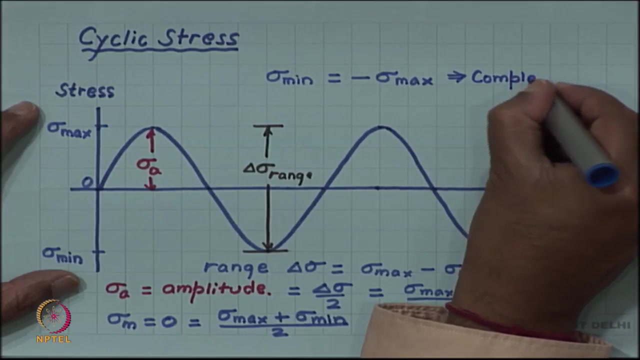 sigma min is equal in magnitude but opposite in sign. sigma max is tensile but sigma min is compressive. So this kind of cycle is called completely reversed cycle. One more parameter we define, called the ratio R, the stress ratio, which is defined as sigma. 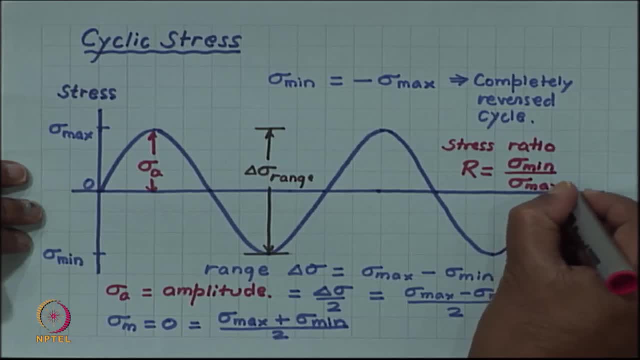 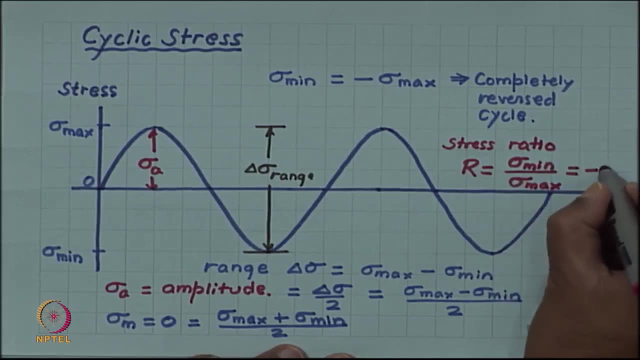 min by sigma max. So in this case, for a completely reversed cycle, we define sigma min by sigma max. This will be minus 1, because sigma min, being compressive, is negative but is equal in magnitude to sigma max, which is tensile and so is positive. So the ratio 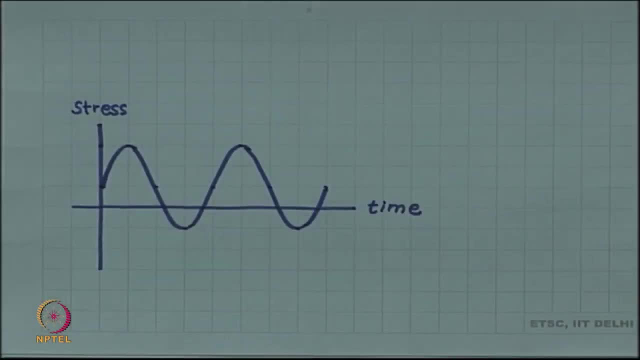 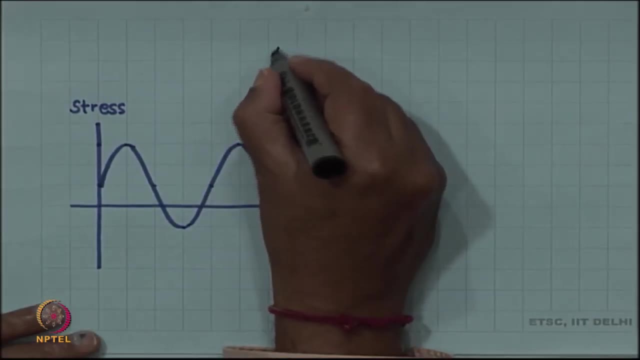 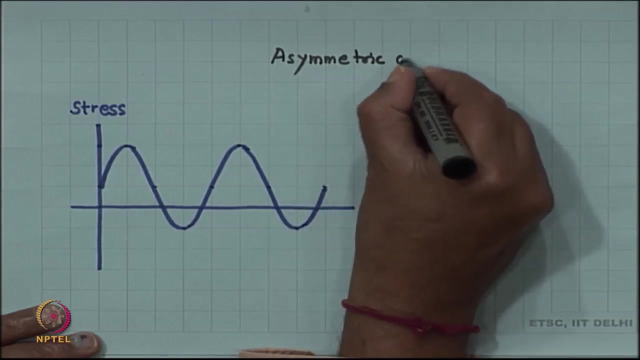 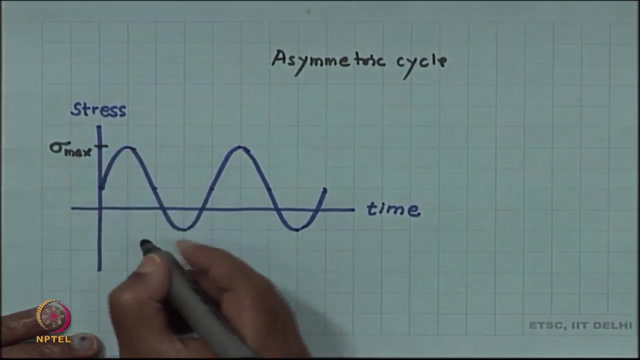 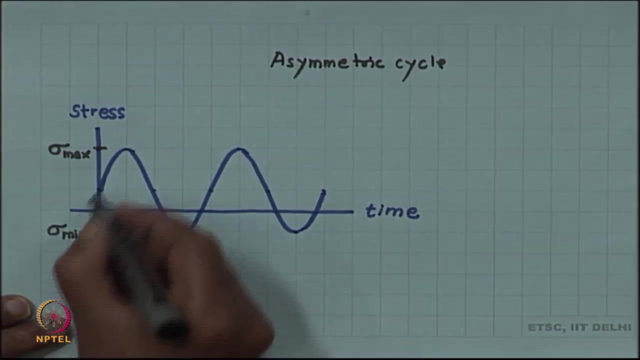 becomes minus 1. That was a completely reversed cycle. This one shows an asymmetric cycle. This one shows an asymmetric cycle where the sigma max and sigma min are not equal in magnitude And thus the mean sigma sigma mean is also equal in magnitude. 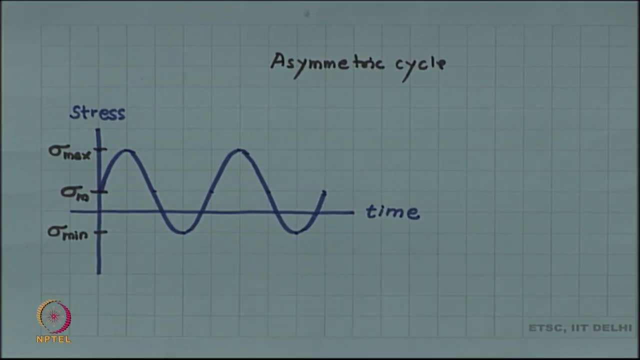 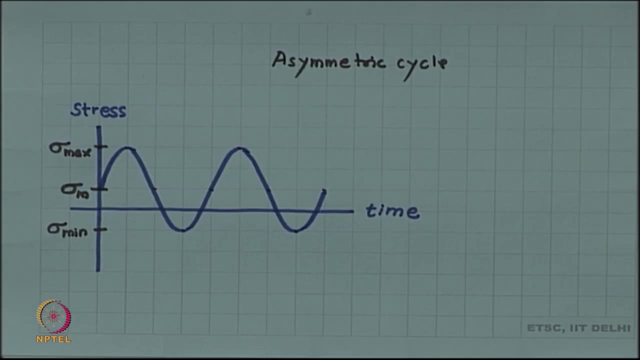 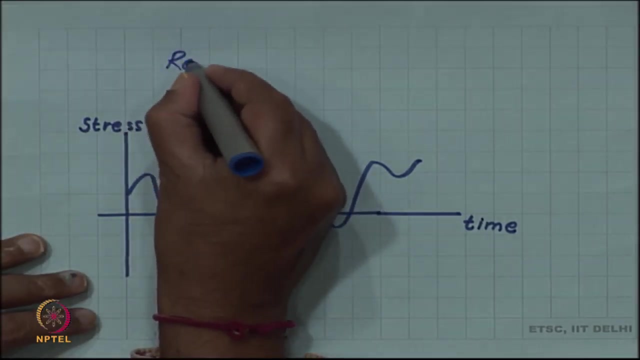 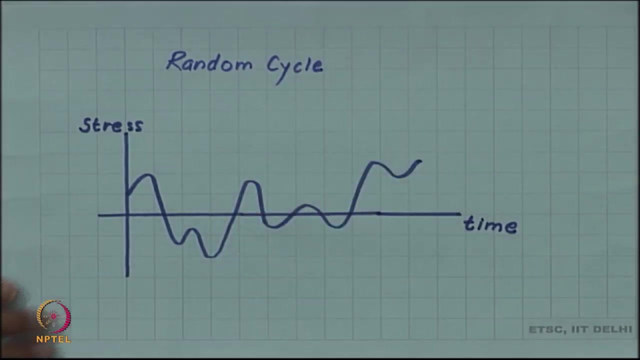 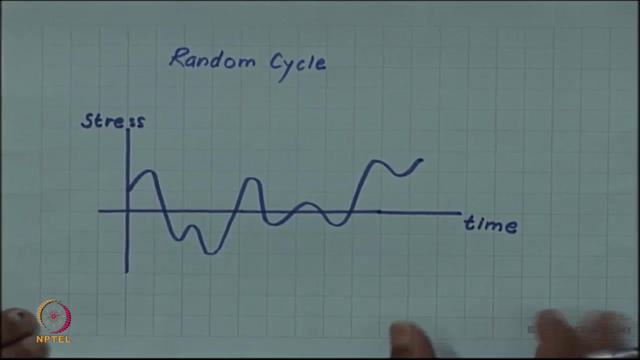 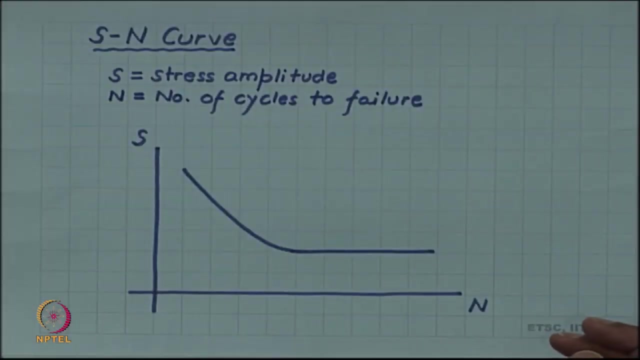 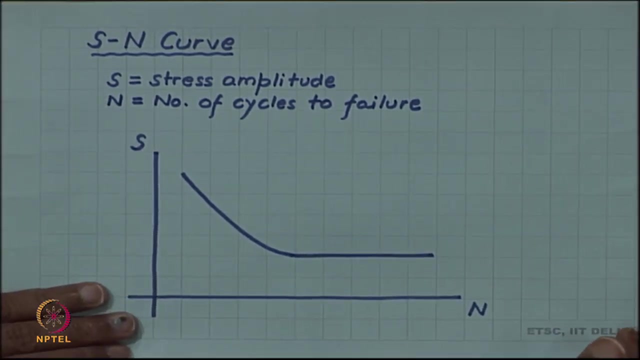 So not 0,, but in this case has some value. We can also have random cycle shown here, which is not defined as a single sinusoidal But it has several maxima and minima varying over time. The result of a fatigue test. a fatigue test is done by alternating the stress amplitude. 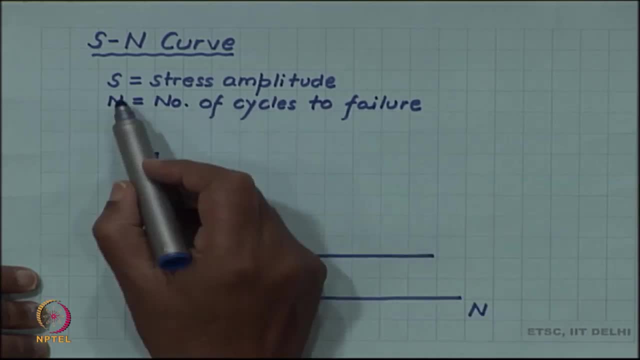 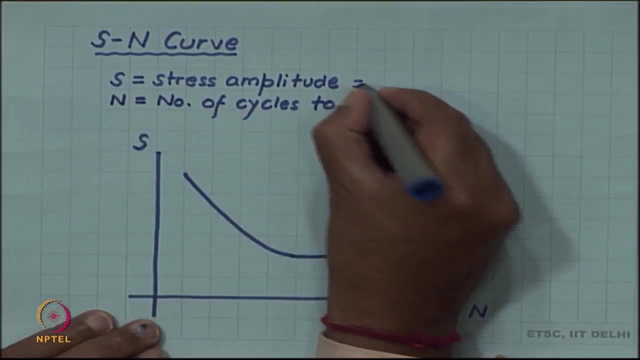 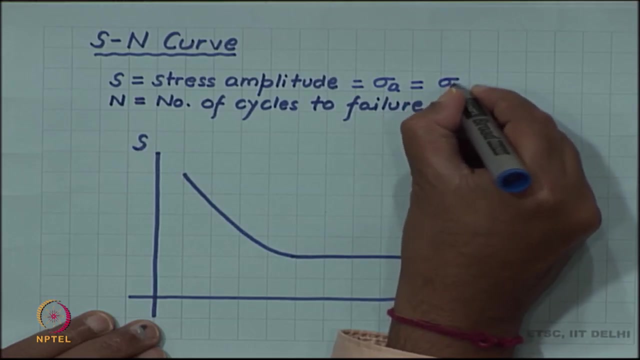 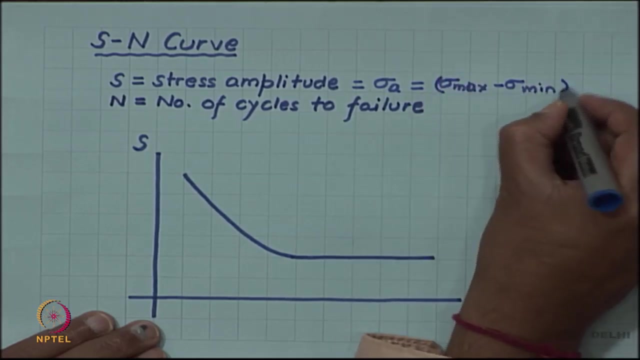 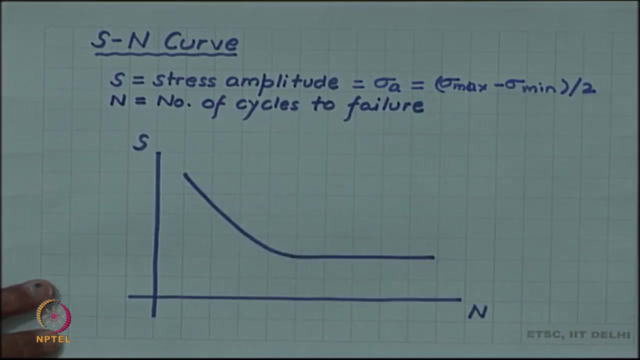 up to the failure of the component. So S gives the stress amplitude which we had in the previous class, denoted by sigma A, amplitude which is sigma max minus sigma min by 2.. The result is shown as an S-N curve, shown here. So S is the stress amplitude, N is the number. 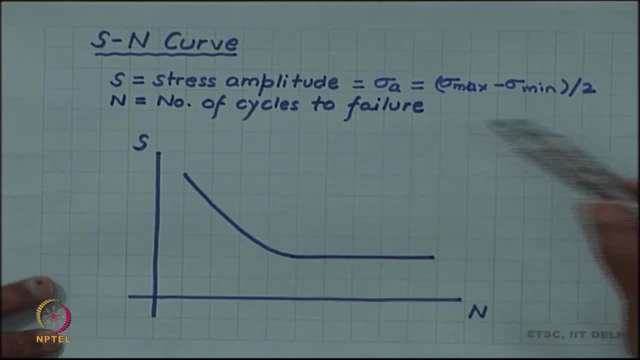 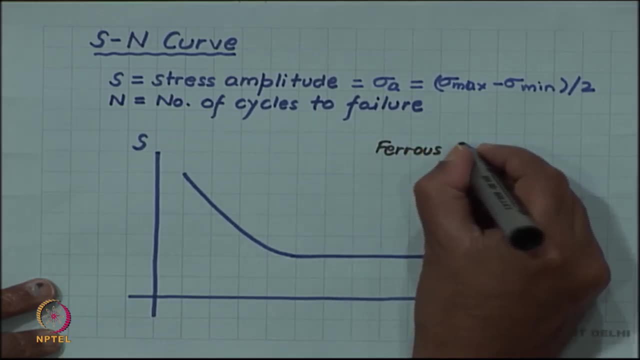 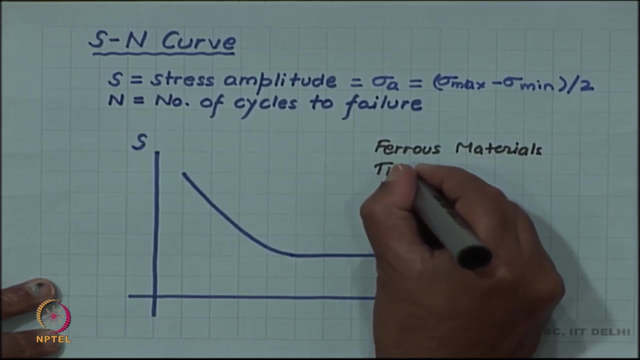 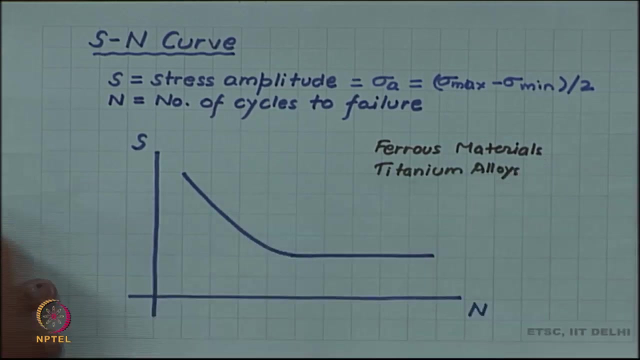 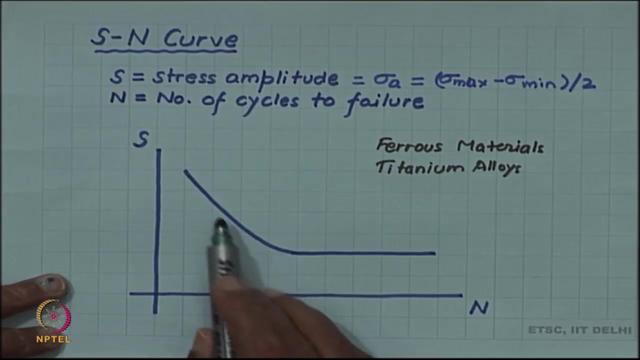 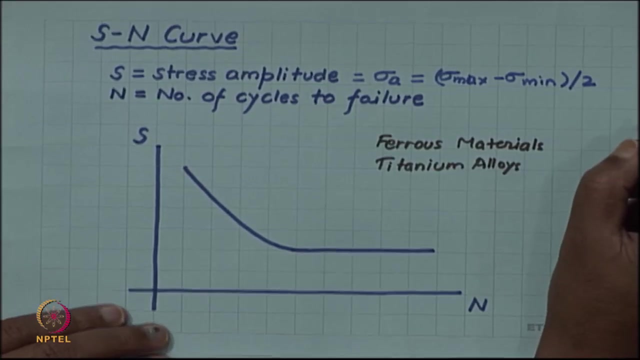 of cycles to failure And for some kind of material, some ferrous material, we have to take some ferrous material also. some titanium alloys show a decreasing number of cycles, decreasing life. So the number of cycles to failure can also be called a fatigue life for that particular stress value. So the life of the component keeps decreasing, or rather increasing, as you decrease the stress amplitude. But beyond a certain point, which we are calling a fatigue limit, we have to take some ferrous material, which is also known as endurance limit. There is no further decrease. there is no failure of the component with any further decrease in the stress amplitude. So there is no fatigue failure below the stress amplitude equal to fatigue limit. 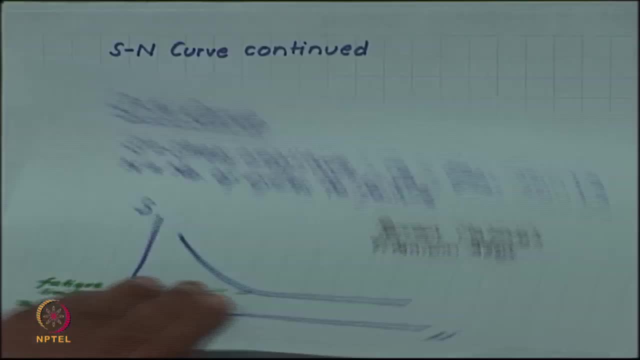 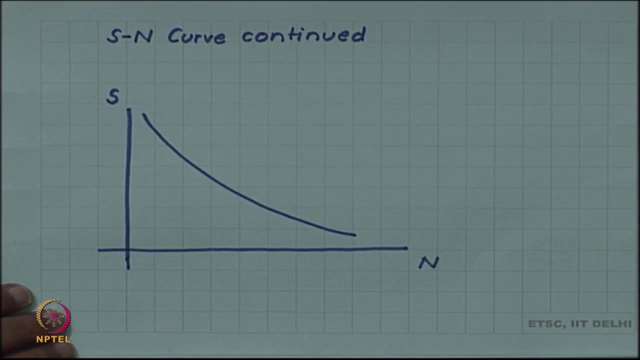 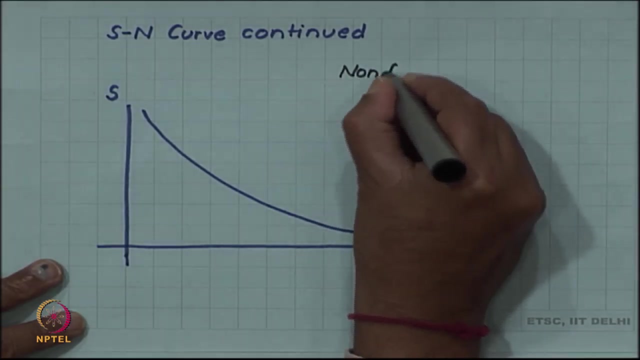 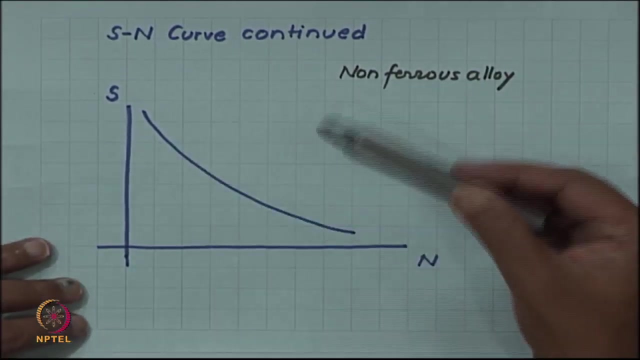 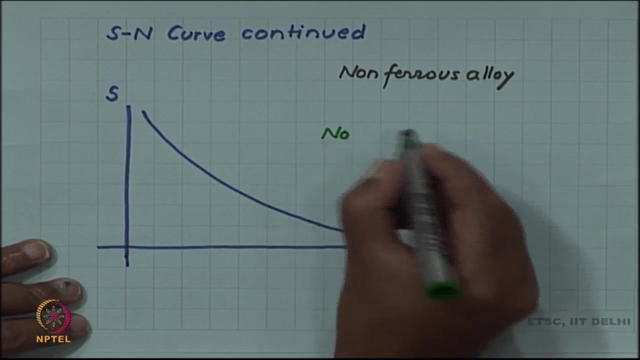 But a different kind of behavior is seen in some non-ferrous material, non-ferrous alloys, where there is no fatigue limit in this case. So this is the non-ferrous material which the curve does not become horizontal. there is no fatigue limit, So no fatigue limit. 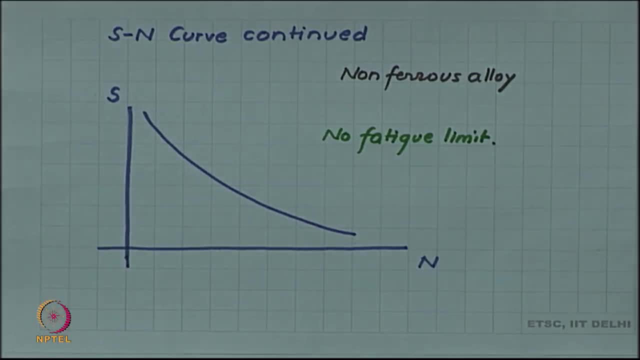 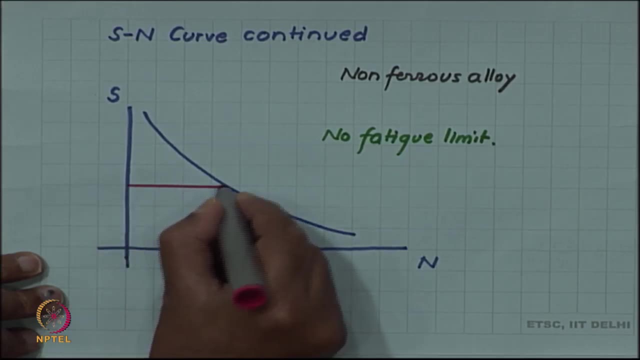 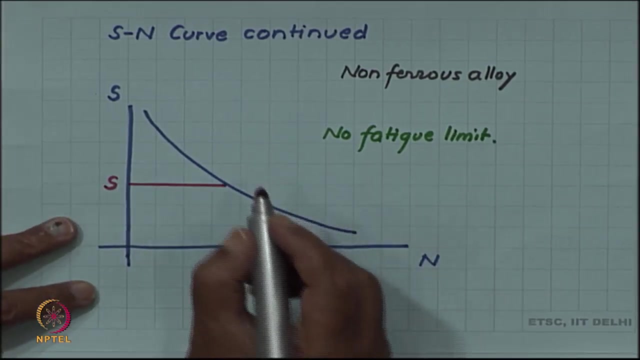 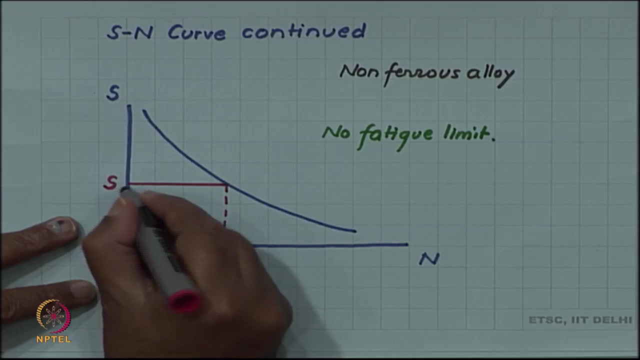 can be specified. So this kind of curve is described by: either: you can have a specified value of a stress amplitude, So let us say that stress amplitude S is a specified value to some value, let us say S 1.. Then NF 1 is called the fatigue life. 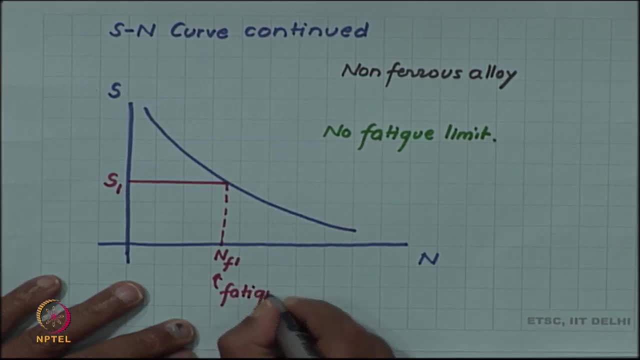 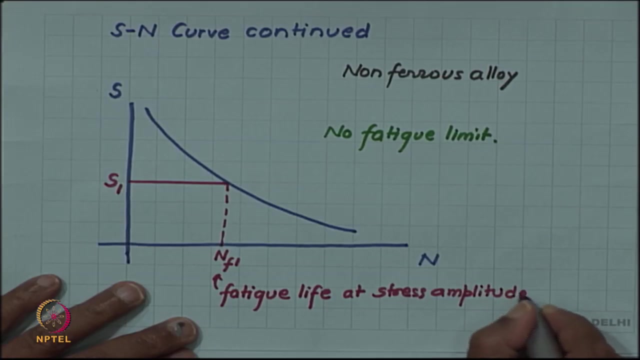 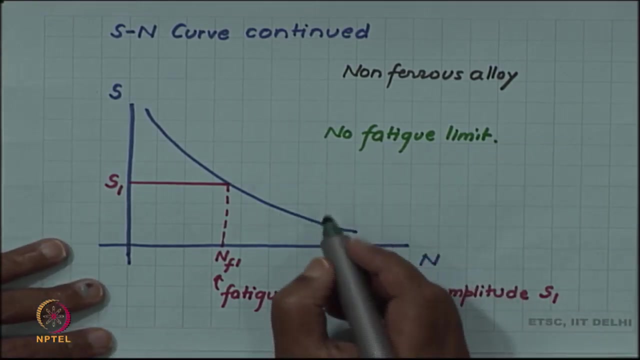 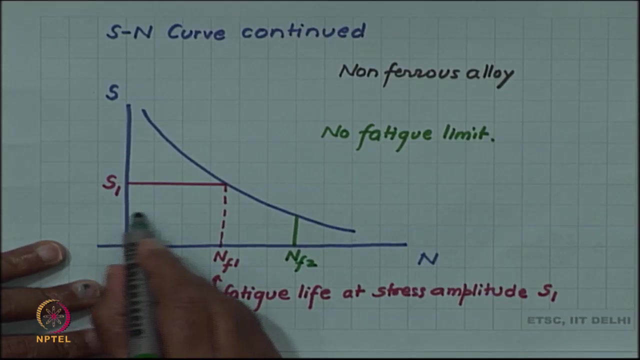 Then this is called a non-ferrous material. This is called, if we look at the non-ferrous at stress amplitude S 1, or you can define a life, let us say N, F, 2 and find the stress amplitude corresponding to that, In this case this: